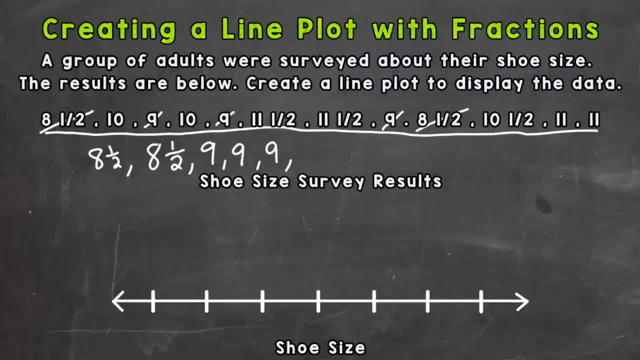 Next would be nine and a half, which it doesn't look like we have any. So we would jump up to ten and we have one, two and that looks like it for ten. So two tens here And then ten and a half, which we have one here. 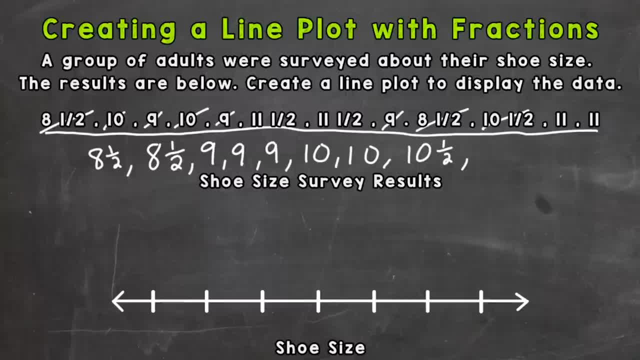 then 11, which we have one, two, and then eleven and a half- we have one two for that as well. okay, so we have our data in order from least to greatest. so I always like to double check to make sure I have everything. so let's see how many people 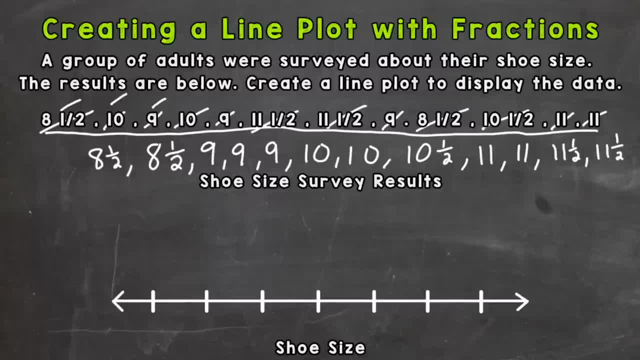 were surveyed. we have one, two, three, four, five, six, seven, eight, nine, ten, eleven, twelve. let's double check our data that we put in order from least to greatest to make sure we have twelve there. one, two, three, four, five, six, seven, eight, nine, ten, eleven, twelve. so we have everything and we didn't repeat anything. so we're. 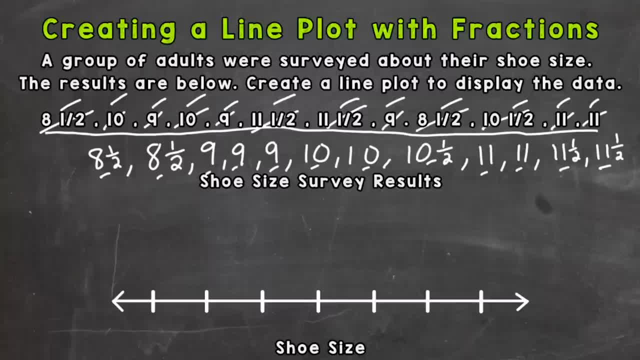 good to go there now. let's take a look at our number line here, and it's very important to set this part up correctly. so we need to take a look at our smallest valued piece of data, which is going to be eight and a half. so that's. 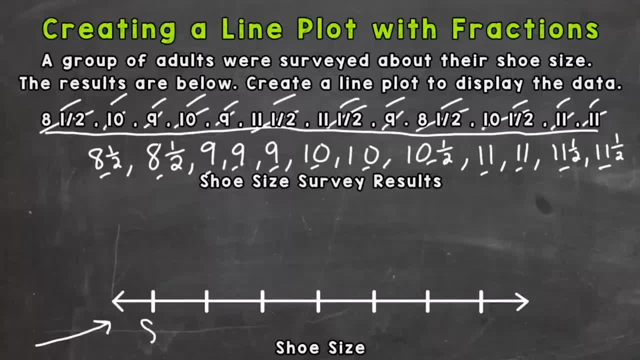 where I'm going to start our number line. so we need to make sure we start with eight and a half. you need to make sure we include everything. so next we need the greatest valued piece of data, which would be eleven and a half. so we need to at least go up to eleven and a half. so eight and a half and it looks. 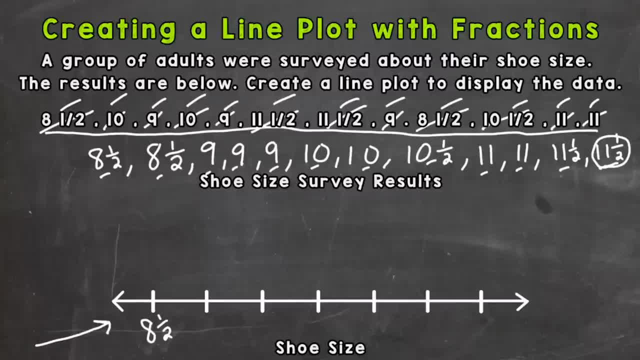 like everything's halves, so we don't have any fourths or eighths or anything like that, so we can count up by halves. so eight and a half, nine, nine and a half, 10,, 10 and a half, 11, and we go up to 11 and a half. 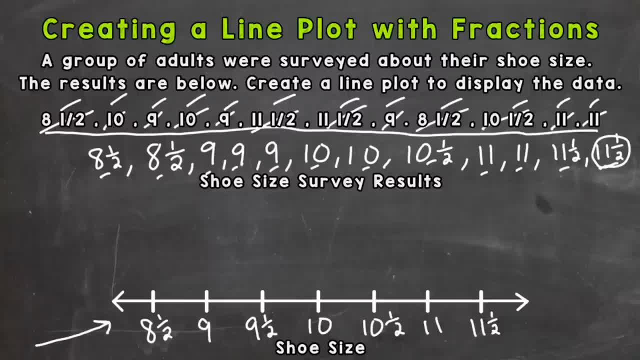 So for this number line, for example, there's no need to go up to 20 for this number line here, You just need to make sure you include the data, the numbers that are in your data. So now we are ready to create our line plot. 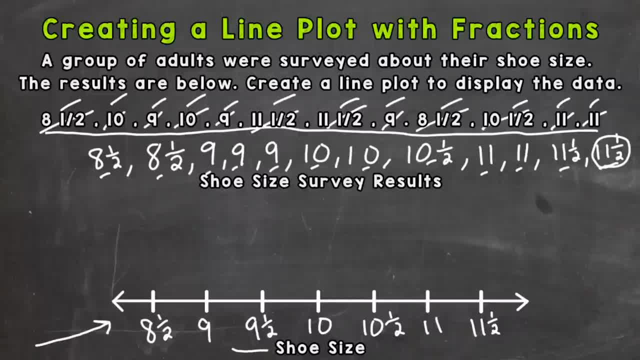 And before we start that I just want to mention down here I have a label It says shoe size. That's my label for what my numbers mean on my number line And then up here I have the title of my line plot. 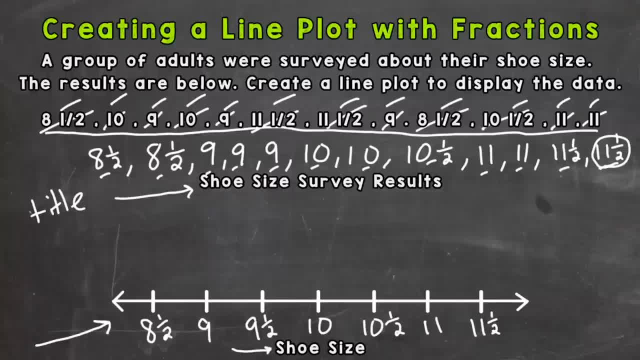 So this is the shoe size survey results And again, shoe size down here at the bottom is my label for what those numbers mean. So we have two, eight and a halves. So I represent each number here with an X on my line plot. 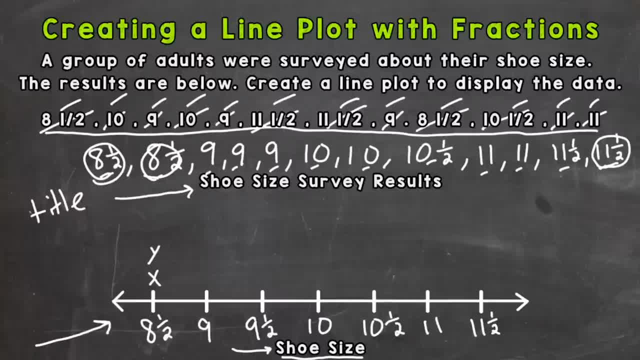 So I would say one, two, and I want all my X's to be around the same size, to the best of my ability. So two, eight and a halves. Then we have one, two, three, nines. So I need three X's to represent those three nines. 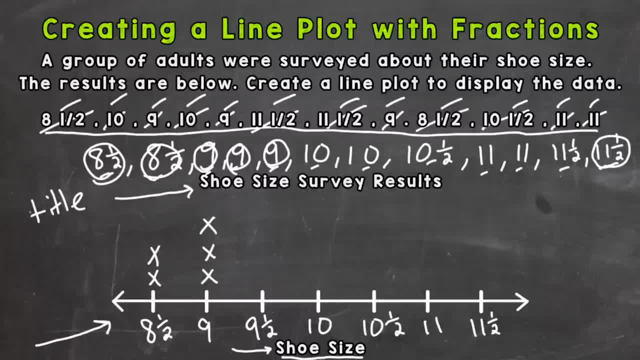 Next nine and a half, which we don't have any. Then we have two tens, One, two, Ten and a half, we have one here, Eleven, one, two And eleven and a half, one, two. And there is our line plot. 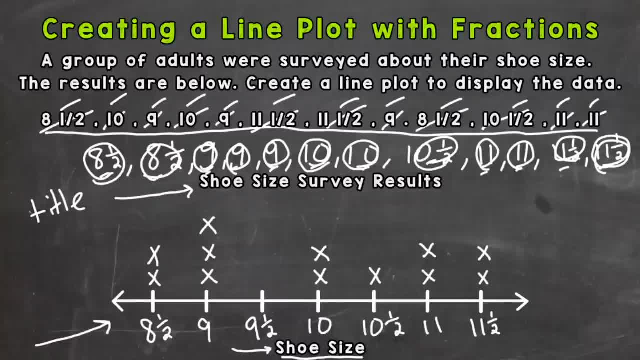 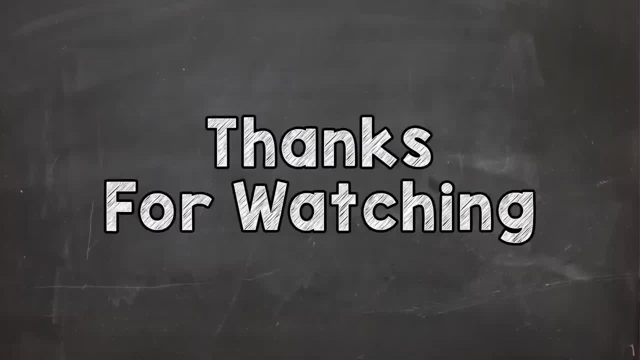 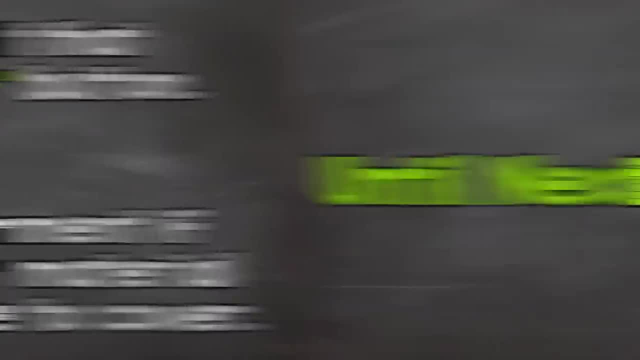 And we have 12 X's down there to represent the 12 pieces of our survey and our data. So hopefully that helped. Thanks so much for watching. Until next time. peace Subtitles by the Amaraorg community.